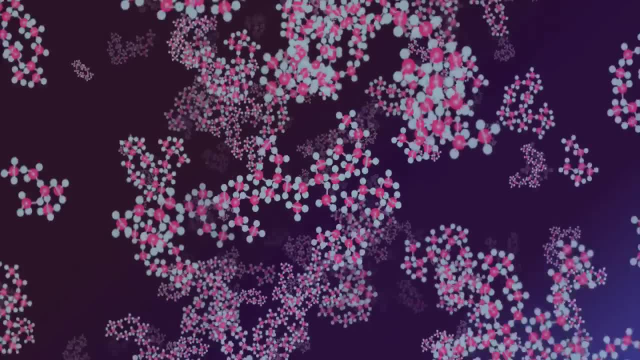 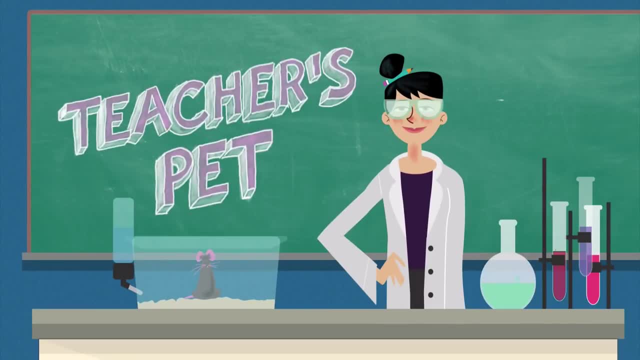 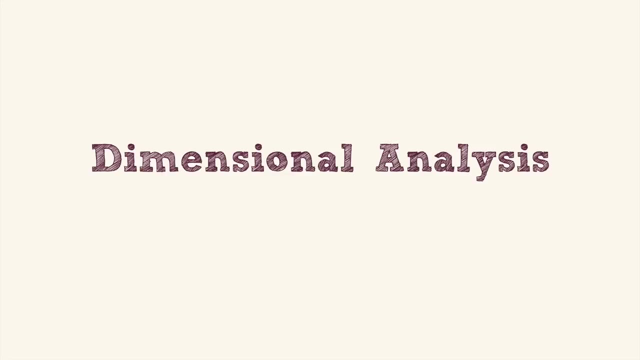 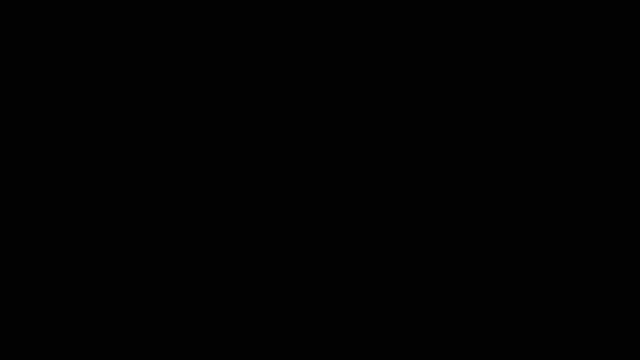 One of my favorite things ever is dimensional analysis. I know that seems crazy, but I'm serious. It's a way to analyze and solve problems using dimensions or units. With dimensional analysis, you can figure out how many size 10 shoes lined up end-to-end it. 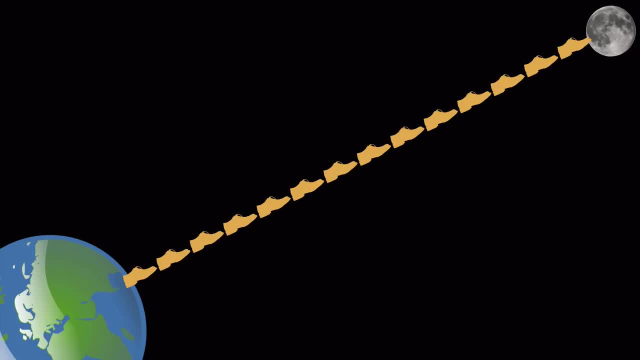 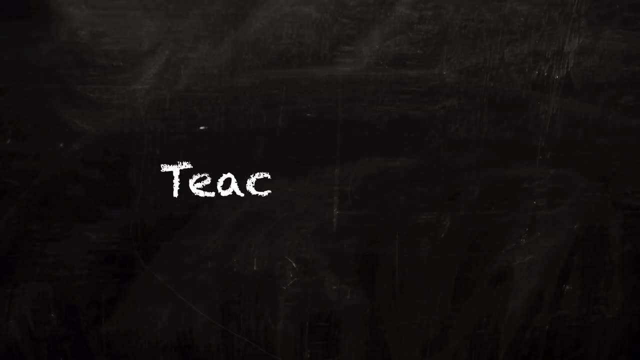 would take to go to the moon, because you totally need to know that, and how many seconds of your life you spend sleeping, or how many formula units of chalk are used to write your name on the chalkboard. It's awesome. Here's the basic idea. Any number multiplied or divided. 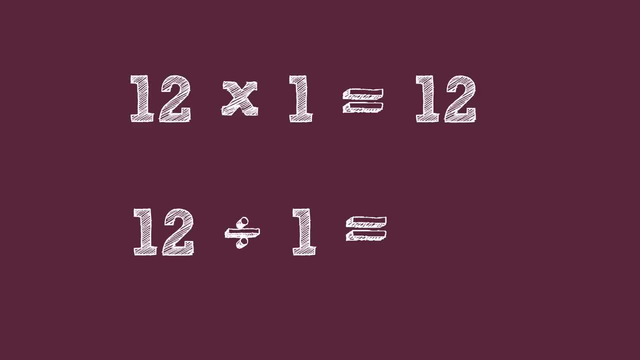 by 1 is still equal to the original number. You could even say that 12 times 3 thirds equals 12, and 12 divided by 3 thirds equals 12.. That's because 3 and 3 are equal to each other and therefore 3 thirds are equivalent to 1.. Now take a conversion like 12 inches: 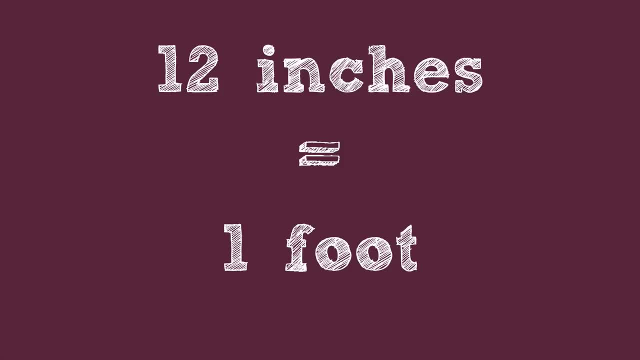 equals 1 foot. You could have 2 feet or 24 inches, and that measurement is really the same. They're equal in the same way that 3 thirds was equal to 1.. So you can write the equal sign like a division. You could also write the equal sign like a division You. 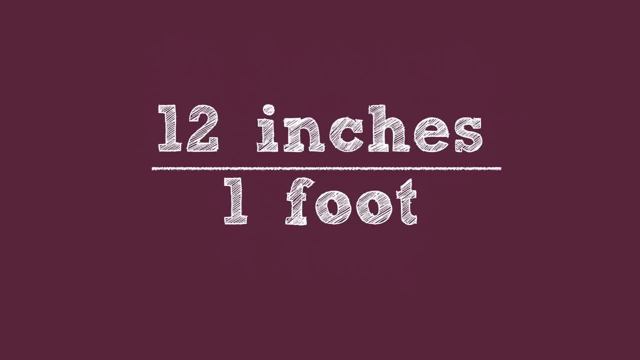 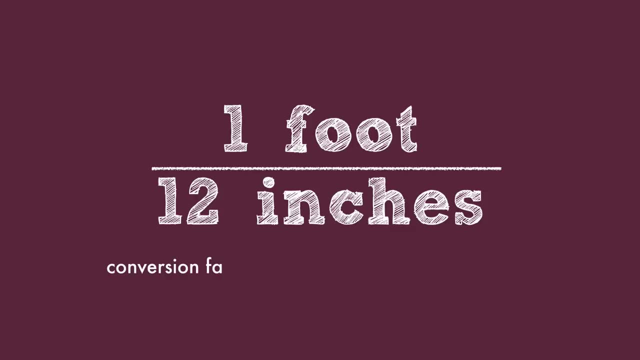 could also write the equal sign like a division sign and read it: 12 inches per foot. But you could also write it the other way and it would still be true: 1 foot per 12 inches. This is called a conversion factor and it's the crux of dimensional analysis: Conversion. 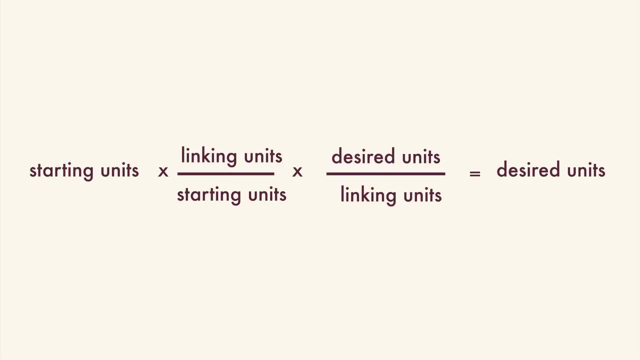 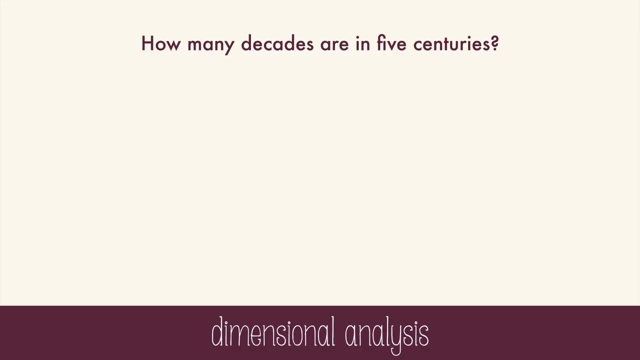 factors allow you to change from one unit to another, to another, and so on, until you get the units you want. So let's try a problem: How many decades are in 5 centuries? Start with what you're given Next in order to get rid of the current unit. 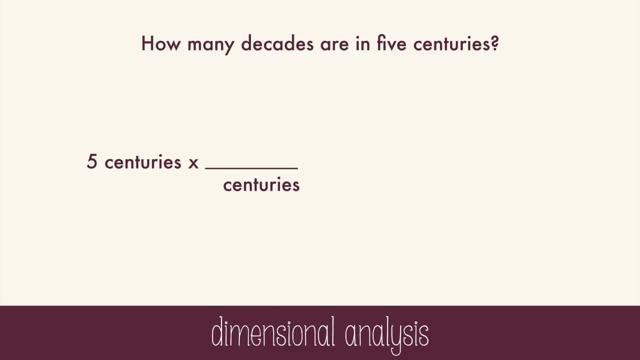 we have to cancel it with the same unit on the bottom of the next conversion factor. Next, you just think of a relationship between centuries and something smaller. In one century there are 100 years. The units of centuries are equivalent, so we can ignore them by crossing. 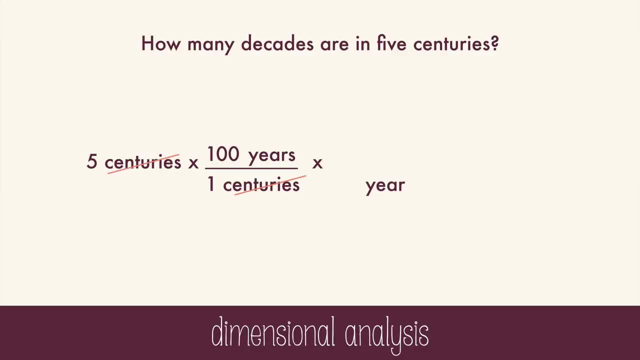 them out Now. we need to get rid of years. So put years on the bottom of the next conversion factor and think of a relationship between years and decades. 10 years makes 1 decade, Years cancel And all that's left is decades. Now just multiply any number on top and divide any 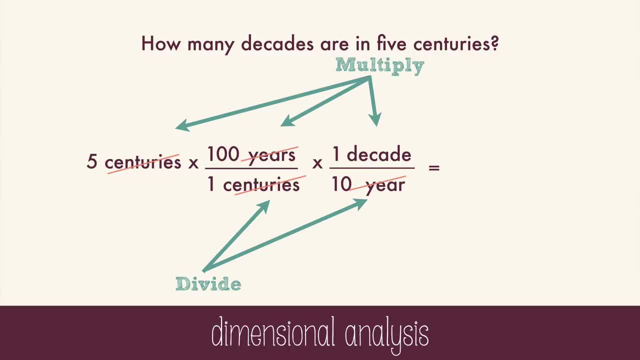 number on the bottom 5 times 100 times 1, divided by 1, divided by 10.. The answer is 50 decades. Now you don't really need to put the ones in your calculator, but make sure the numbers on top are all multiplied and the numbers on the bottom are divided. Let's try another. 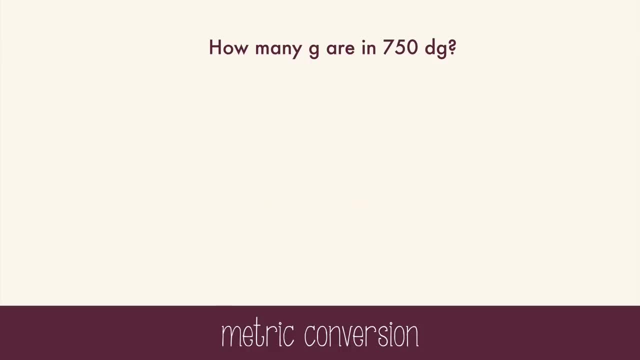 How many grams are in 750 decigrams? First you need to know your metric prefixes. I use the mnemonic: King Henry died unexpectedly drinking chocolate milk. Do remember kilo, hecto, deca, unit, deci, centi and milli. These decrease by a factor of 10. 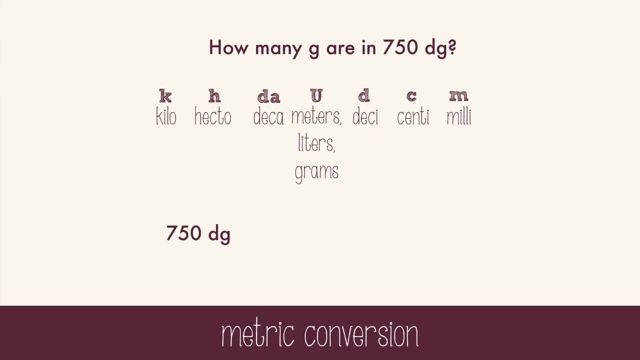 as you go from left to right, Start with what you're given. Now let the units guide you. Decigram will have to be on the bottom to cancel and grams will have to go on top. Now give the larger unit a value of 1. And, with metrics, see if you can get the units. to be on the bottom. Now, the unit that's on the bottom is the unit that's on the top. The unit that's on the bottom is the unit that's on the bottom, And the unit that's on the bottom is the unit. 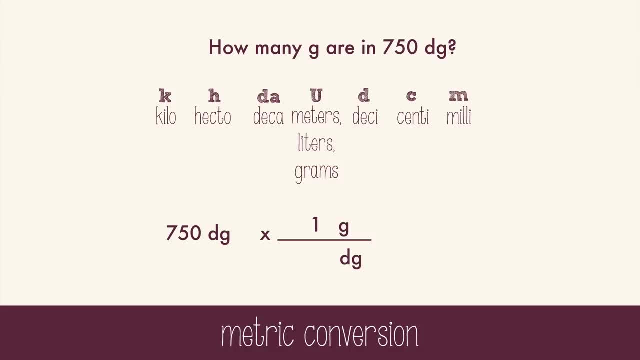 that's on the bottom, See how much smaller the unit is. by multiplying, We move from deci to the base unit in one move, so it's just times 10.. Now calculate the answer and you get 75 grams. Let's do one last problem: Convert 7.21 grams per cubic centimeter to kilograms. 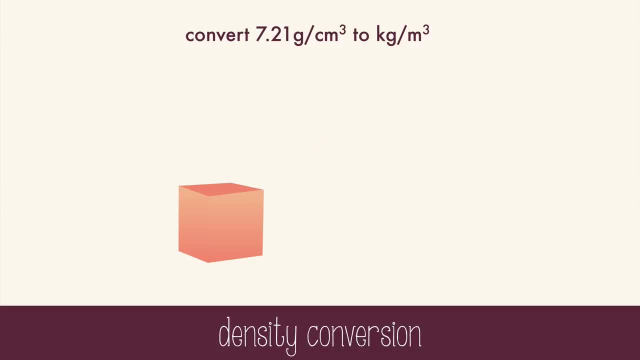 per cubic meter. We're changing two things here. First, start with what you're given. When you say per, it's like drawing the fraction line. Now you could choose either grams or centimeters to change. next, It doesn't matter, but I'll 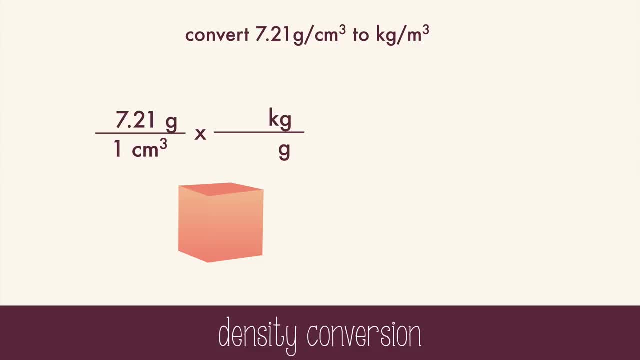 just go with grams. Grams on the bottom, kilograms on top. Kilograms are larger, so they get a 1. Use the mnemonic to see the amount of difference. Grams to kilograms is a change of 1,000 times, Then grams cancel.